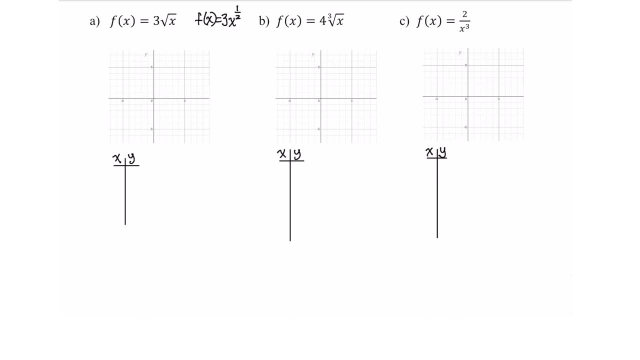 So I can write it in the form of f of x is equal to a times x to the n, where I've got a number times x to a number power. Now, how do I go ahead and graph this? Well, when I look at it, it's a little bit more comfortable to graph it in the format that it was originally presented. 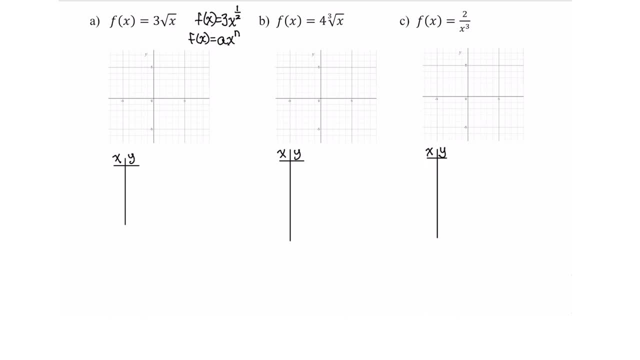 The f of x is equal to 3 times the square root of x. Now remember, Over the reals, the square roots are only defined for non-negative numbers, So my domain of this is including 0 and then off to positive infinity. 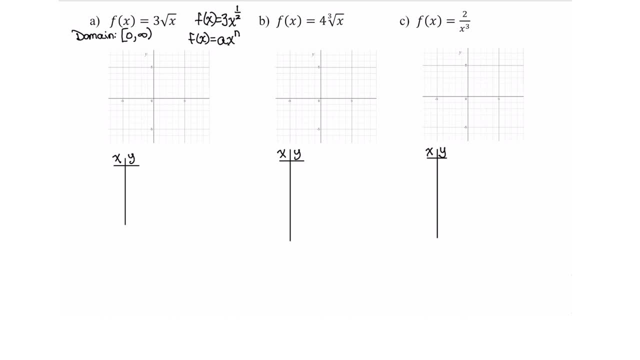 And that helps me figure out what values I want to plug into a table, to get some coordinate points on the graph and then to graph it. So since my domain is starting at 0 and off to infinity, I will substitute 0 in for x. 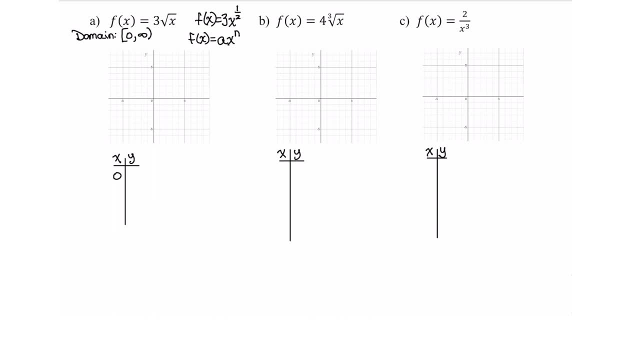 And then, looking at the function, it's the square root of what I put in for x. So I would love to put in numbers that are perfect square numbers, so that I have nice points to graph. So let's also put in 1.. 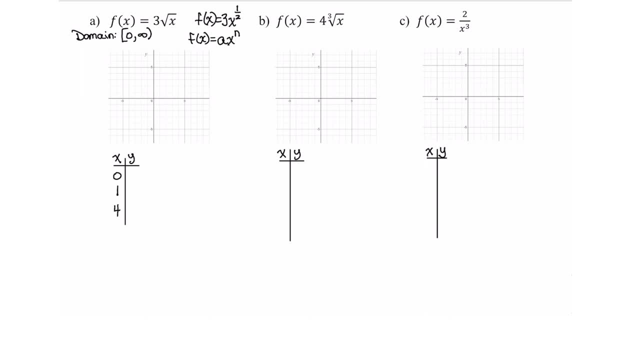 And then after that let's put in 4. And a lot of times students will ask: well, how many values should you put in? And you want to get like 3 to 5 of anything that's not linear, Of what. 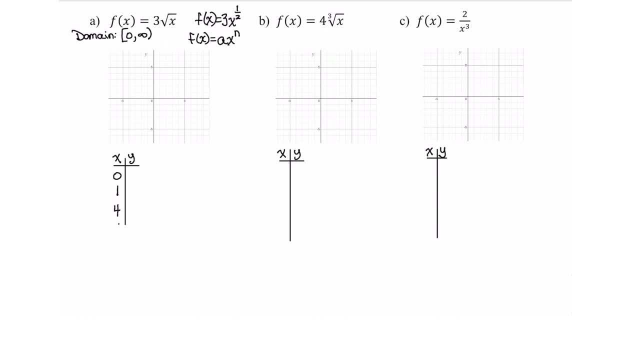 Well-chosen points, So let's go ahead and also put in 9 to get just another point there. So when I'm looking at these, if x is equal to 0, this would be 3 times the square root of 0.. 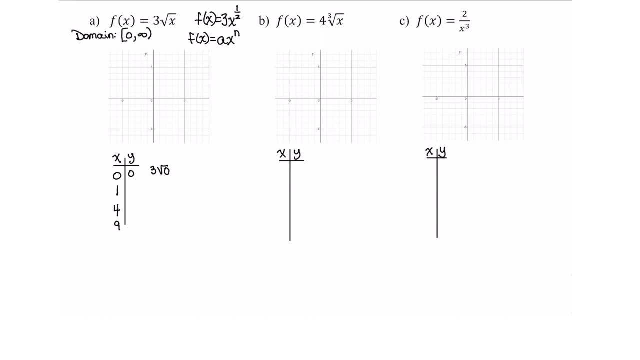 Well, square root of 0 is 0 times 3 is 0.. How about if x is 1?? Well, that would be 3 times the square root of 1.. Square root of 1 is 1.. 3 times 1 is 3.. 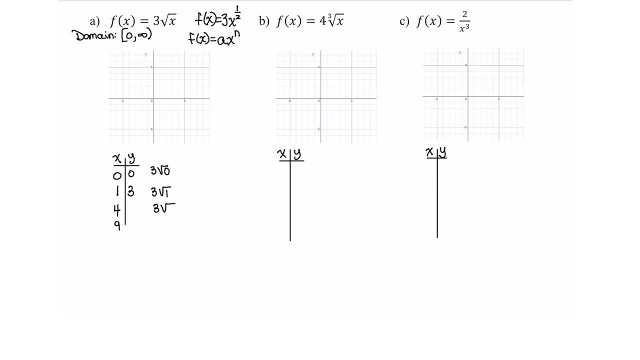 How about if x is 4?? That would be 3 times the square root of 4.. Square root of 4 is 2.. 3 times 2 is 6.. And then, finally, if x is equal to 9, I have 3 times the square root of 9.. 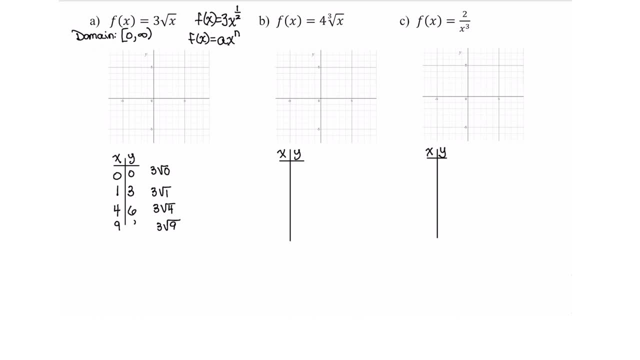 Square root of 9 is 3.. 3 times 3 is 9.. So now, looking at these, I can plot the points. I have 0,- 0.. I have right 1 up 3.. I have right 4 up 6.. 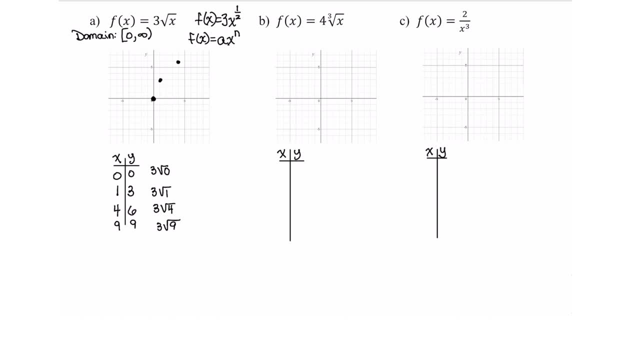 And then I have right 9.. So here's 5,, 6,, 7,, 8,, 9, just on the outskirts there, And then a little bit off the graph if I go up 9. Then, connecting these, I get my graph. 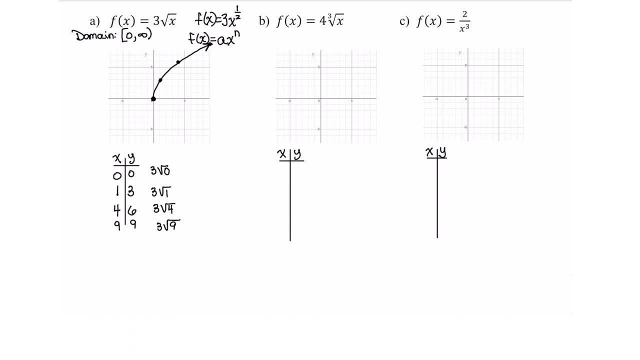 All right, How about the next one? f of x is equal to 4 times the cubed root of x. Well, cubed roots are valid for all real numbers, So my domain for this one is from negative infinity to infinity. So I do want to represent both the negative values input for x as well as positive. 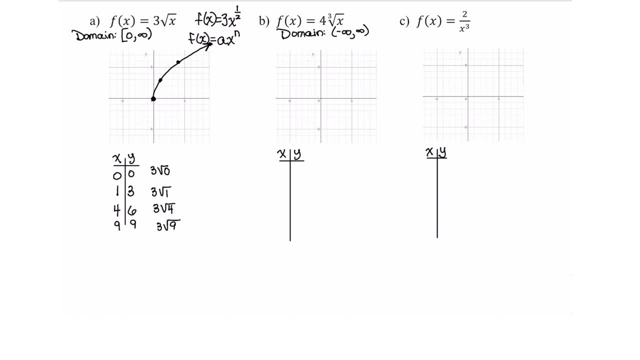 So, then again, knowing that this, looking at what the function does, it is the cube root of whatever I put in, So I want to put in perfect cube numbers, And also this can be written as: 4 times x to the one-third power. 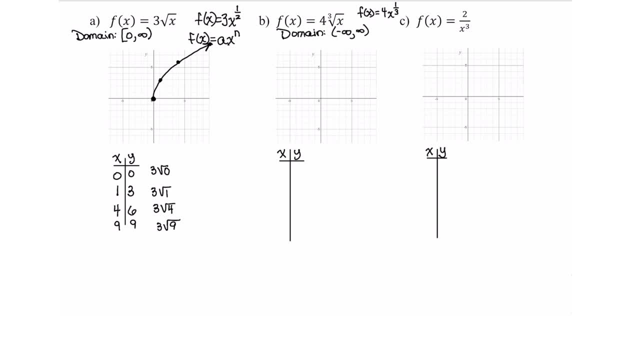 So again, it is also a power function. Now, perfect cube numbers. Perfect cube numbers would be like 0,, 1,, 8. And then also negative 1 and negative 8.. And I like to put them in the x column, from smallest at the top down to biggest at the bottom. 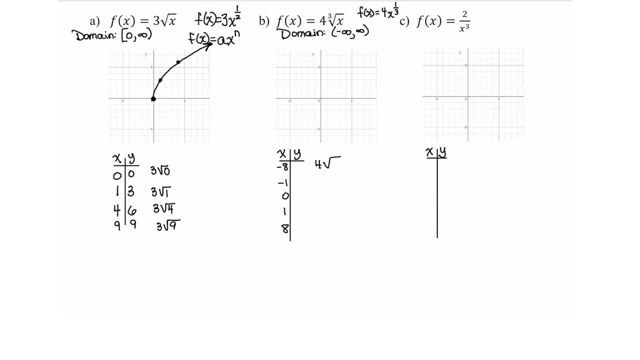 All right. So now let's calculate our values 4 times the cube root of negative 8.. Well, the cubed root of negative 8 is negative 2.. 4 times negative 2 is negative 8.. And then negative 1.. 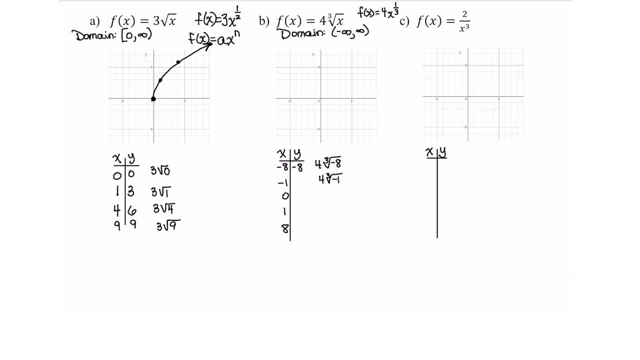 4 times the cubed root of negative: 1.. 4 times the cubed root of negative: 1.. 4 times the cubed root of negative: 1.. Cubed root of negative: 1 is negative: 1.. 4 times negative: 1 is negative 4.. 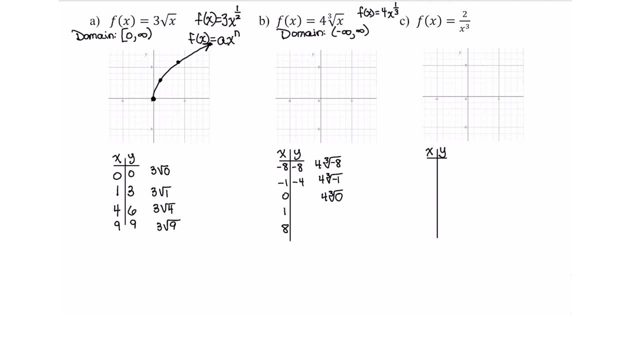 Plugging in 0 for x: Cubed root of 0 is 0.. 4 times 0 is 0.. Plugging in 1 for x: Cubed root of 1 is 1.. 4 times 1 is 4.. 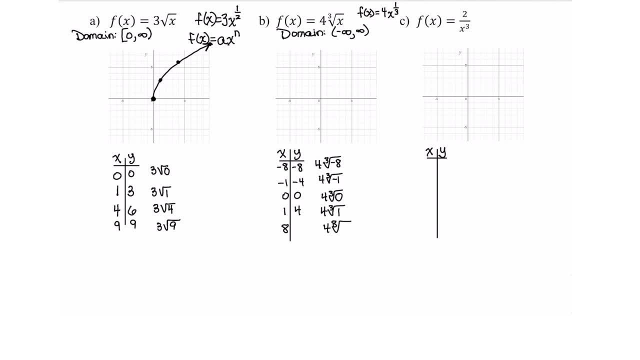 And then plugging in 8 for x, Cubed root of 8 is 2.. 4 times 2 is 8.. So notice here that if I just would have plotted the points negative 8, negative 8, 0, 0, and 8, 8,, 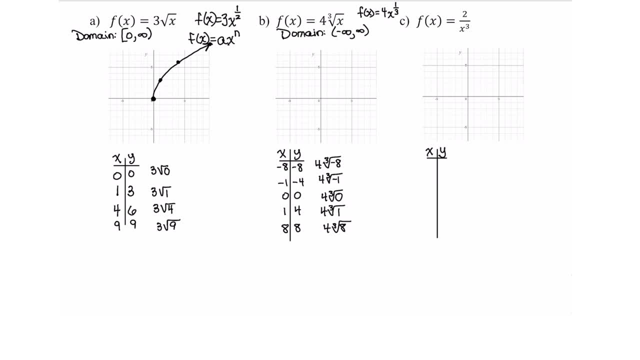 I would have had a misrepresentation of what the graph actually does. So that's why you want to make sure you get a lot of points that you can generate and plot so that you get a better indication of what the graph looks like. So negative 8, negative 8 is a little bit off my graph, but it's about down here. 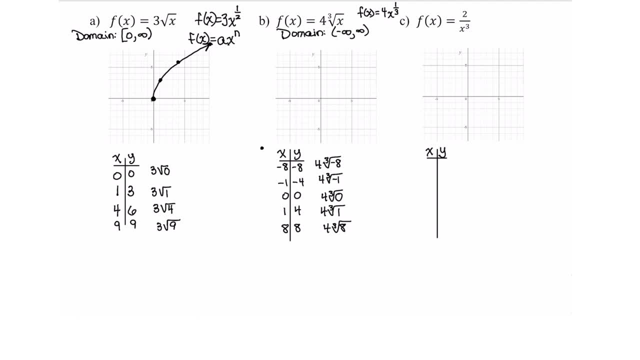 And then negative: 1, left, 1, down, 4 is here, And then 0,, 0,, 1, 4,. so right 1, up 4, and then 8, 8.. So 5,, 6,, 7,, 8, and then up 5,, 6,, 7,, 8.. 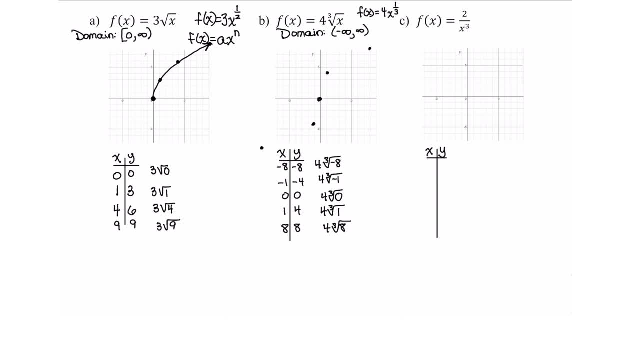 So there, And as I then connect these, I get that graph. All right then. lastly, we have f of x is equal to 2 over x to the third. I can write this function as 2 times x to the negative 3 power. 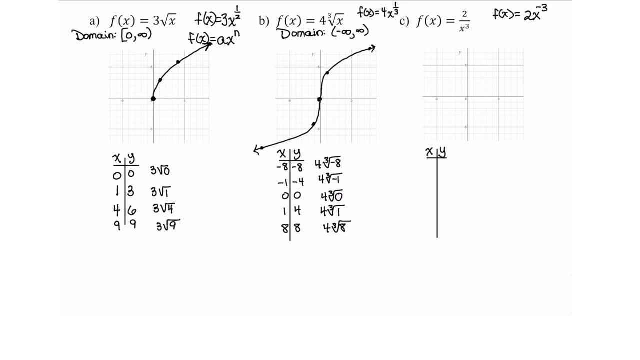 So it is a power function, but its exponent is negative 3. So it is one that does something a little bit different than when I have non-negative exponents. Now, the domain of this is all reals except 0, because we can't plug 0 in for x. 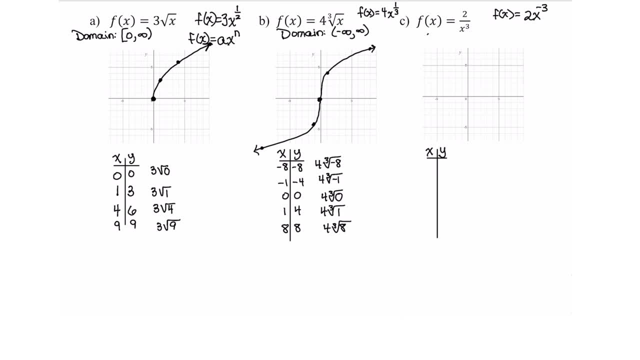 I would get a 0 in the denominator of the fraction. So this is negative infinity to 0, union 0 to infinity, with parentheses at the 0 to show that I cannot use that as a value on my table. So here we are going to plug in different values of x. 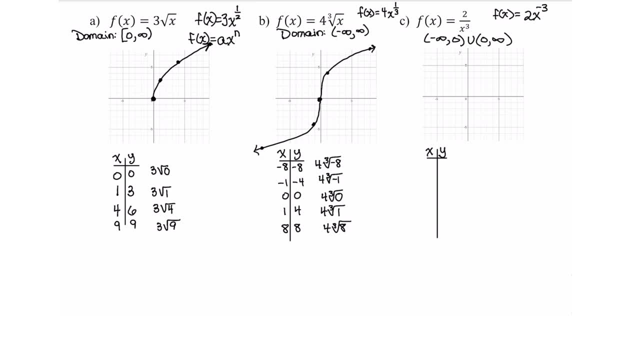 and I'm going to cube them and take 2 and divide by that cube And I can't put 0 in here. So I'm just going to show that I can't do that on my table. But I could put, let's say, negative 1, half or negative 1, positive 1 half, positive 1.. 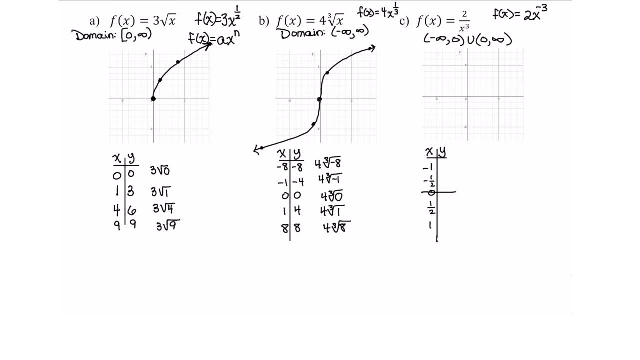 those sorts of values for x, and then definitely you could put more in, but these are the ones that I'm going to show as examples. right? so plugging in negative 1, I have 2 divided by negative 1 cubed. well, negative 1 cubed is. 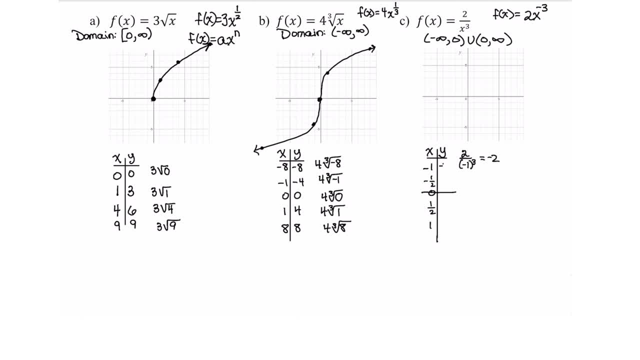 negative 1. 2 divided by negative 1 is negative 2. now be careful on plugging in the negative 1 half in the denominator. you're gonna have 2 divided by negative 1. half cubed is negative 1 over 8. but when you divide by a fraction you have: 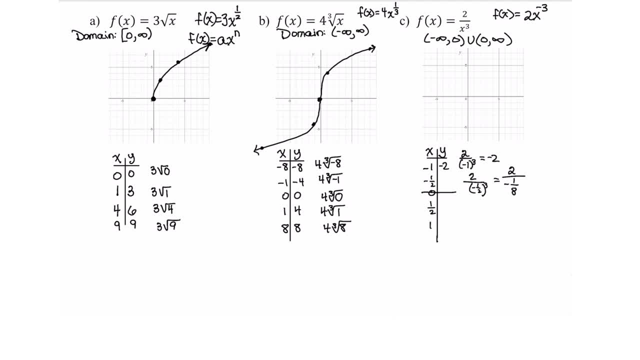 to keep the numerator the way it is and multiply by the reciprocal of the denominator. so this is actually going to give me 2 times a negative 8, which is a negative 16. we can't plug 0 in. when we put 1 half in, I have 2 divided by 1 half. 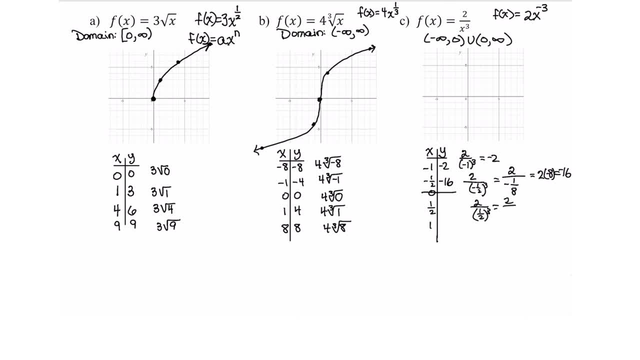 quantity cubed, which is 2 divided by 1, eighth, which gives me positive 16, and then, when I substitute 1 in for X, I have 2 over 1 cubed. 1 cubed is 1, 2 divided by 1 is 2. so 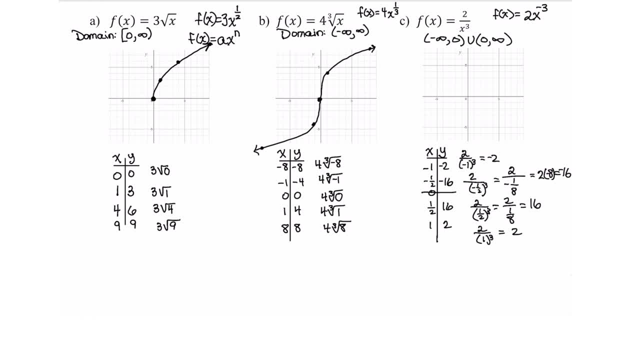 I have negative 1, left 1 down 2, and I have left 1 half down 16, so it's like way down here. and then I have right 1 half up 16, so like way up here, and then right 1 up 2. 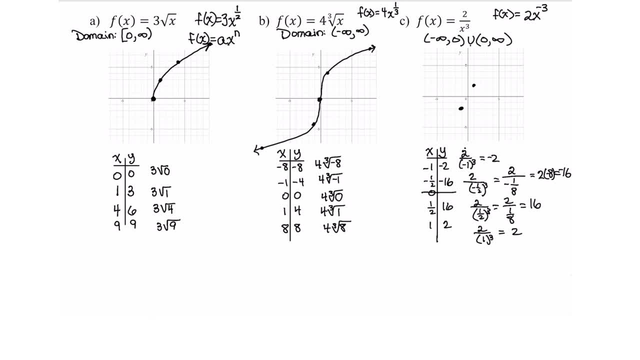 and if you were to put in- let's just see what's happening on this other side. let's, for example, put in 4, then that would be 2 over 4 cubed, so that's 2 over 64 or 1 over 32. and if I put negative 4 in, I would have negative 1 over 32. so as 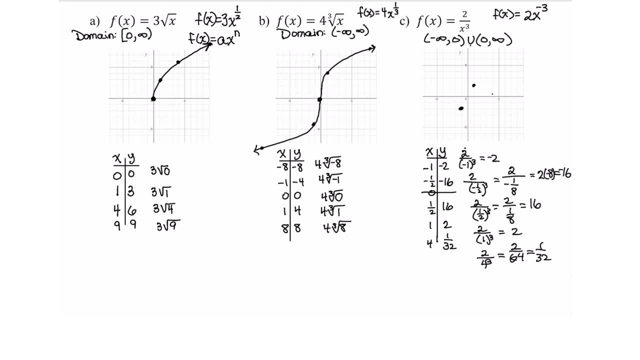 I'm at 4. I'm just really really close to the x-axis but above it. and then if I were to put in negative 4, I would be really really close to the x-axis but on the negative side. so as I connect these, I get this graph. so there are three different examples of how you can get. 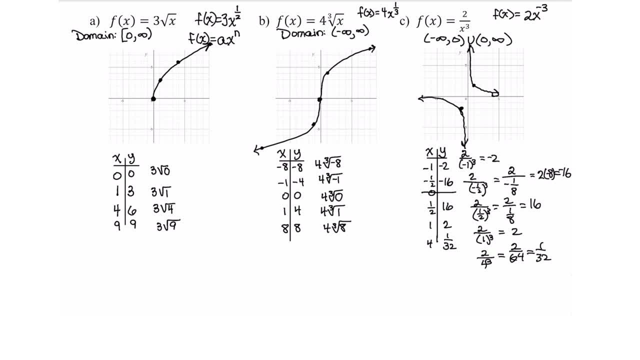 the graph of power functions if their exponents are different than non negative integers. 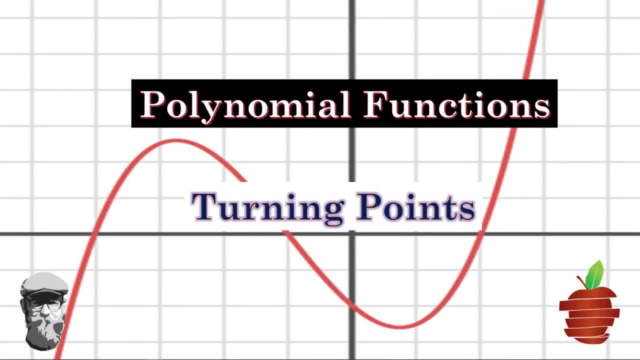 Hello and welcome to the Bearded Math Man's YouTube channel. In this video, we're going to be talking about our third lesson in polynomial functions. We're going to be introducing you to some new concepts that are related to something called turning points. 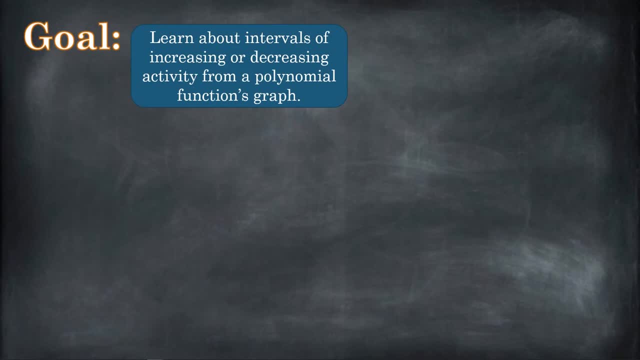 So our goals are as follows: We need to learn how to determine if an interval on a polynomial's graph is increasing or decreasing. I'm going to show you what that looks like. We're going to relate it to slope. We're also going to learn what a turning point is and what a turning point is not. 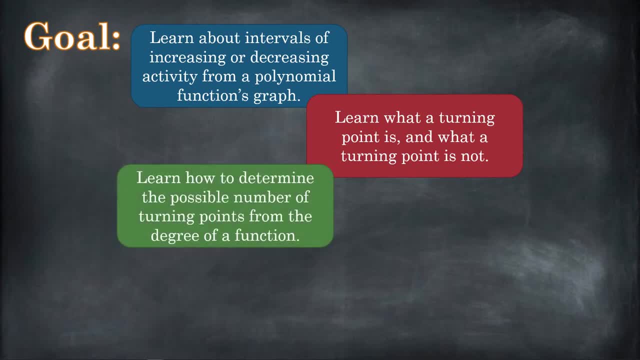 And we're going to learn to determine the number of possible turning points of a function by looking at its degree. Now, as always, I've got some notes that are typed up in practice problems. Those are all hosted on my website, thebeardedmathmancom, and I will put a link to the specific materials related to this video in the description below.